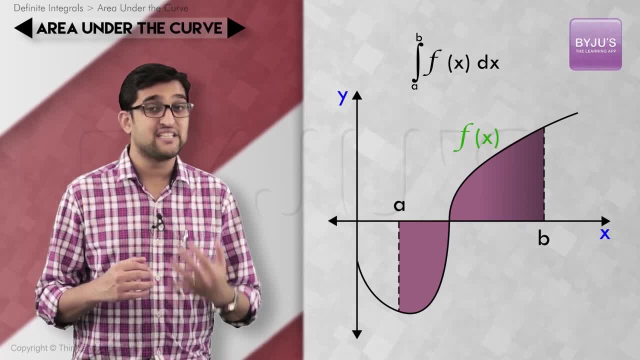 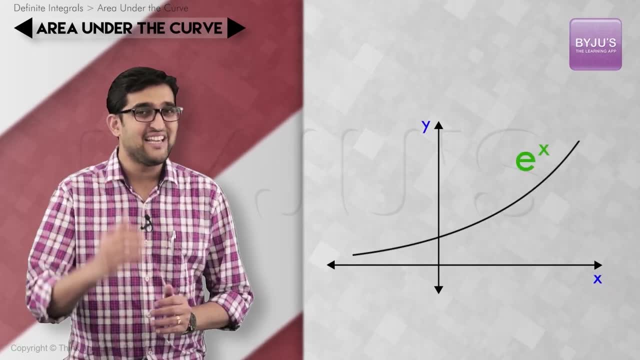 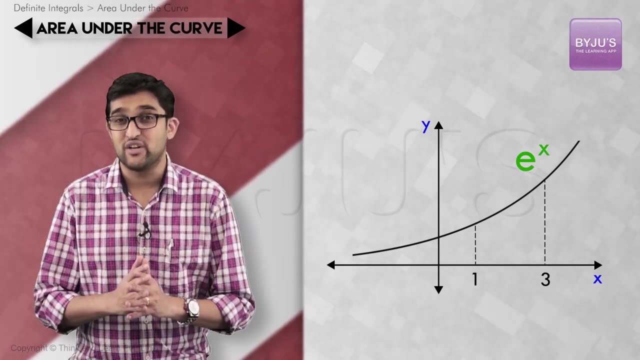 the fact that we need to calculate separate integrals each time the value of the function changes. sign, For example: consider: area bounded by the curve: y is equal to e raised to x, x-axis, and the lines x is equal to 1 and x is equal to 3.. As you know, this plot is always. 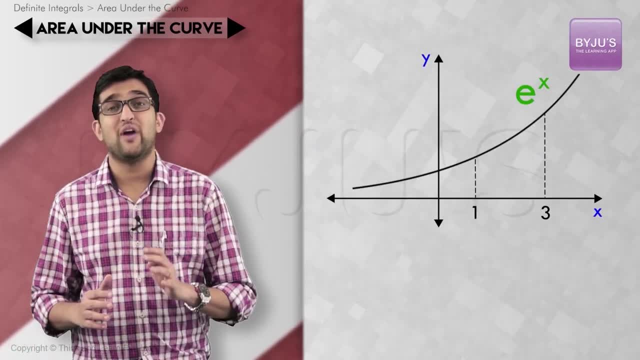 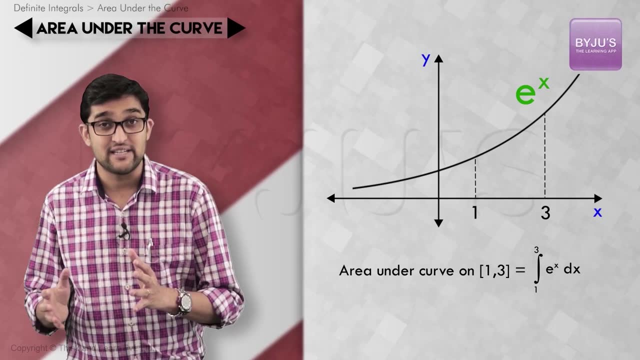 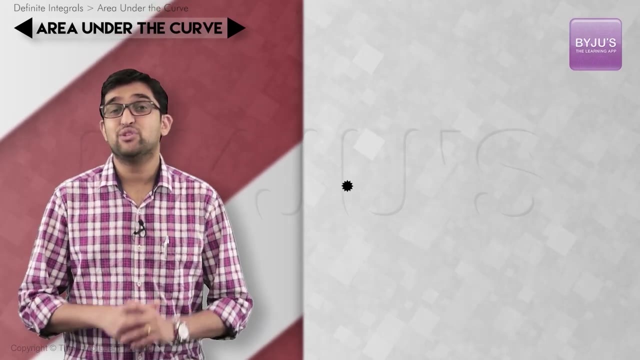 positively valued. So we don't need to draw the plot to arrive at the graph, since the integral, that's integral a to b, f of x, dx, will provide us with the area required by applying appropriate limits on the functions in the equation. But imagine a case where we need to find the area between a and b And the function is: 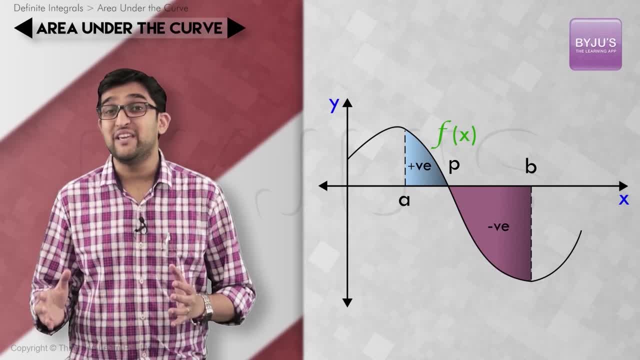 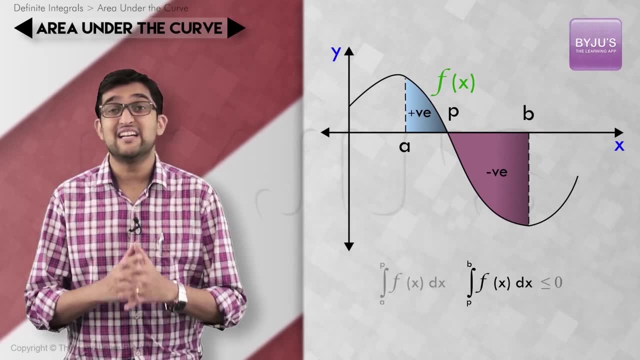 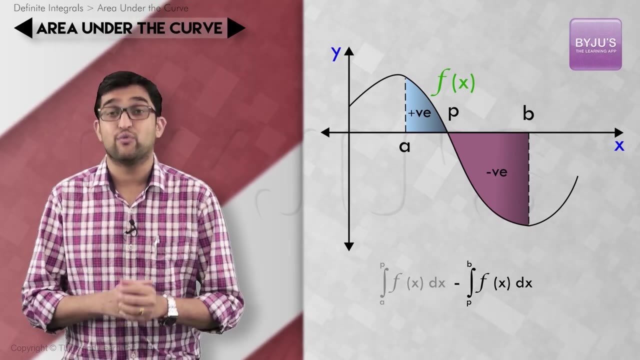 positive from a to p and negative from p to b, where b, of course, lies between a and b. Here, as the integral from p to b turns out to be negative, we should put a negative sign to get the absolute value of our area calculation. 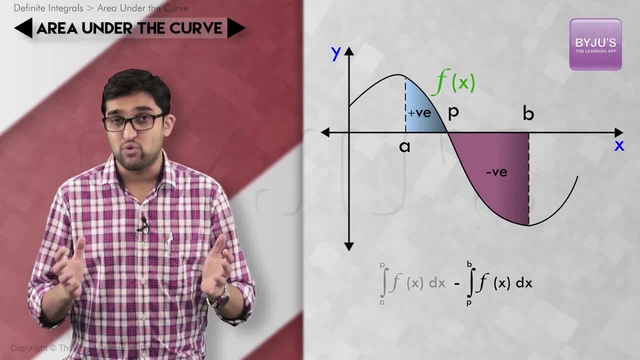 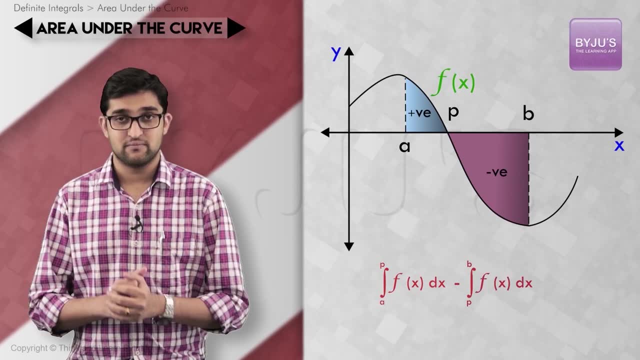 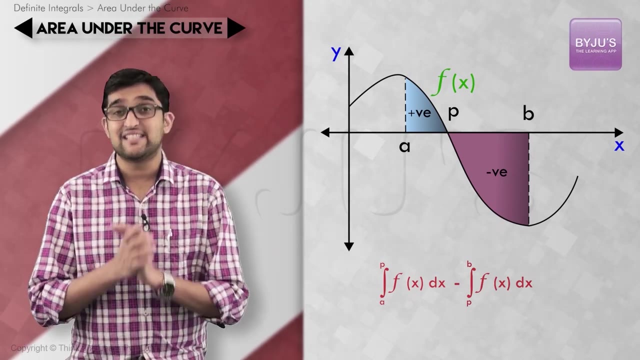 We can arrive at the formula as: area is equal to integral a to p, f of x- dx, minus integral p to b f of x- dx. So what will be the general form for finding the area between the curve y is equal to f of x, x-axis and the abscissus a and b. 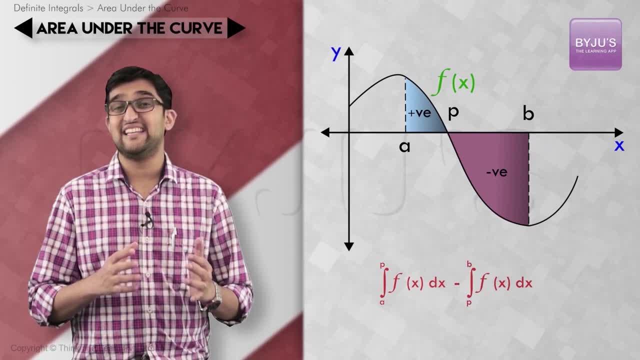 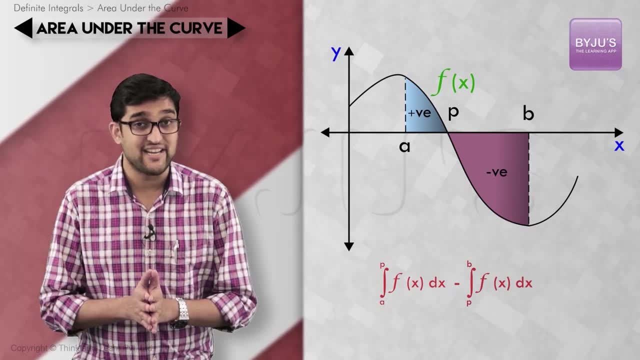 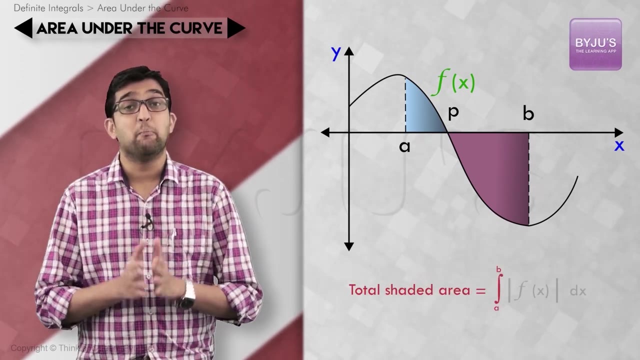 Since we want the absolute area values for all area sections, it will be the sum of absolute value of area. If we find the area of shaded regions, or formally stating, the expression will look something like this: Total area is equal to integral a to b, modulus of f of x- dx. 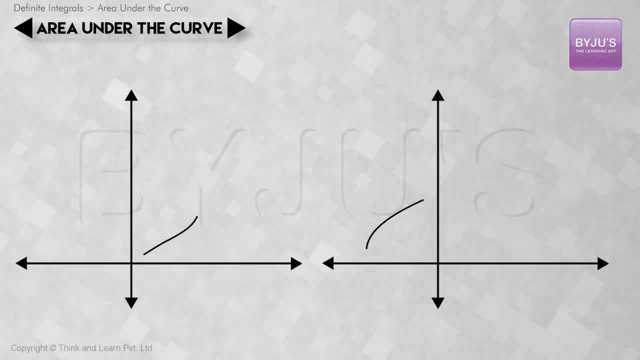 Now we go to the second possibility of finding the area between the plot- x is equal to g- of y y-axis between the ordinates a and b. It would come intuitively to you if you have comprehended the previous case properly. So let's start with the first possibility.